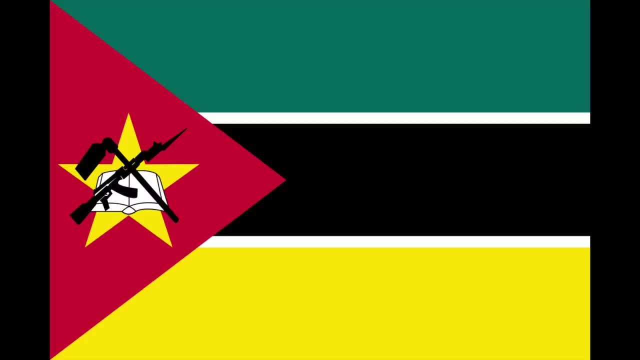 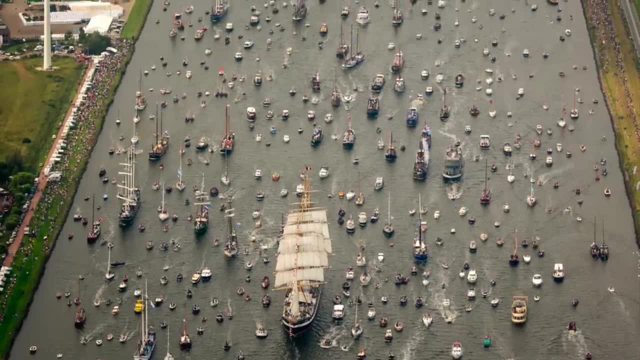 The flag of Mozambique includes the image of an AK-47, and is the only national flag in the world to feature a modern rifle. Amsterdam has a maritime event that occurs every five years, called Sail Amsterdam, where tall ships from all over the world come to participate in the event. 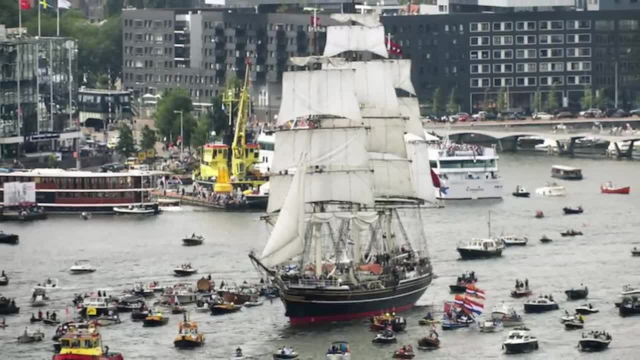 This event was organized for the first time in 1975 to celebrate the 700th anniversary of Amsterdam. The flag is a national flag that is non-quadrilateral in shape. The flag of Mozambique is the national flag of Mozambique. Between Russia and the US state of Alaska lies the 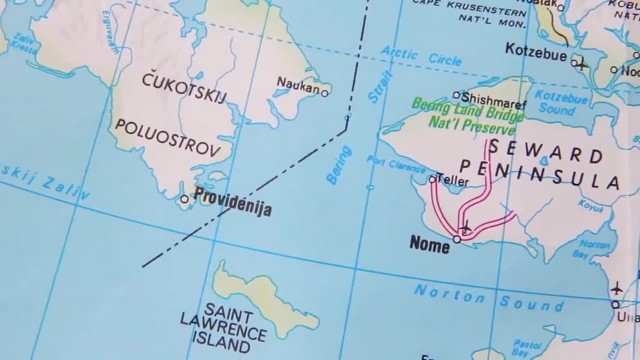 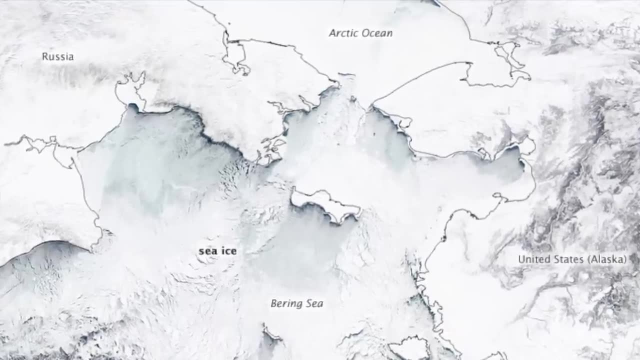 Bering Strait. When it freezes up in the winter, you can journey across, with 3.8 kilometers being the shortest end. In 2006,, two adventurers set out from Alaska to cross the frozen path on foot. It took them 15 days before they were detained in Russia for violating immigration laws. Located in the rainforests of Indonesia is the world's largest flower, the Roflasia arnoldi. It can grow to be 3 feet across and weigh up to 15 pounds. The number 4 is widely avoided in many East and Southeast Asian countries. 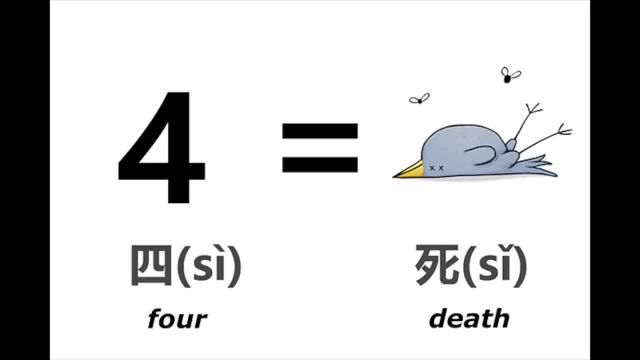 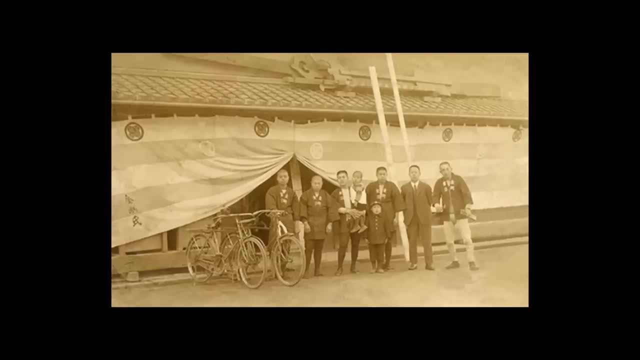 as it often sounds too similar in their respective native languages for the word for death. Often times, the 4th floor and number 4 for house numbers are skipped. Japan is home to the oldest company in the world, and Japan also has no melt ice cream. 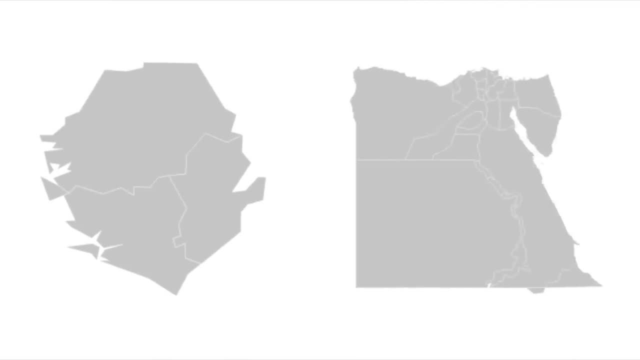 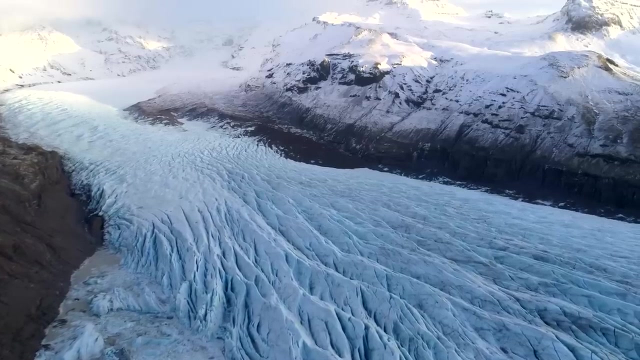 Sierra Leone is the roundest country on earth and Egypt is the squarest. Iceland is often called the land of ice and fire. About 11% of the country is covered in glaciers. At the same time, it is home to 32 volcanic systems. 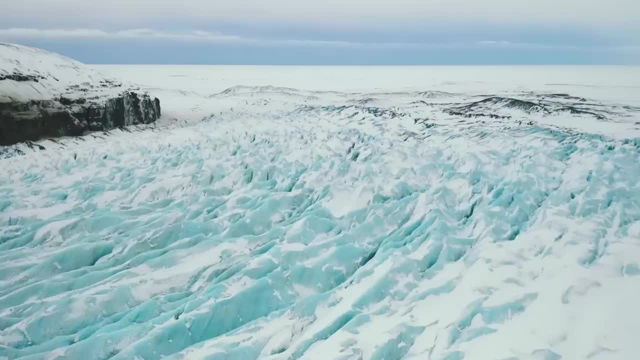 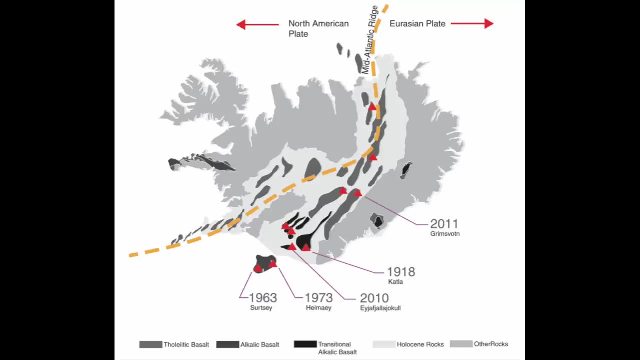 encompassing around 130 volcanic mountains. Thanks to the cold temperatures and lack of shallow ponds, Iceland also does not have mosquitoes. Iceland sits where the Eurasian and American tectonic plates meet. These plates are moving apart, causing the country to grow by about 5 cm per year. 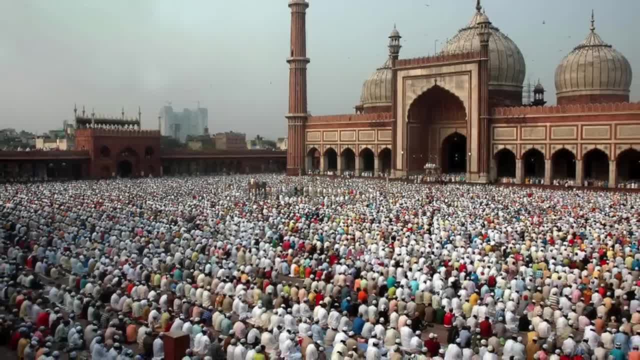 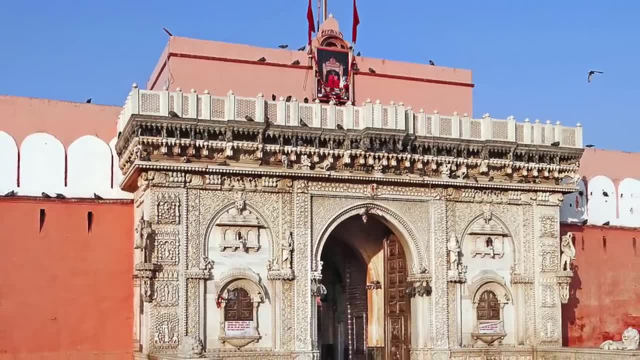 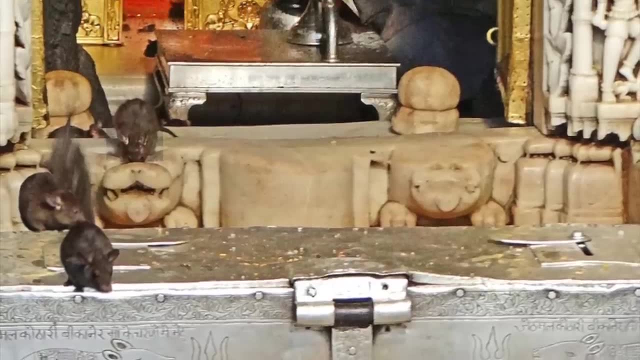 You can actually swim between these two plates. India has over 300,000 mosques and 2 million Hindu temples, One of which is home to 25,000 rats. Legend has it that Karni Mata, an incarnation of a Hindu warrior goddess, implored Yama, the Hindu god of death, to revive her son who had drowned. 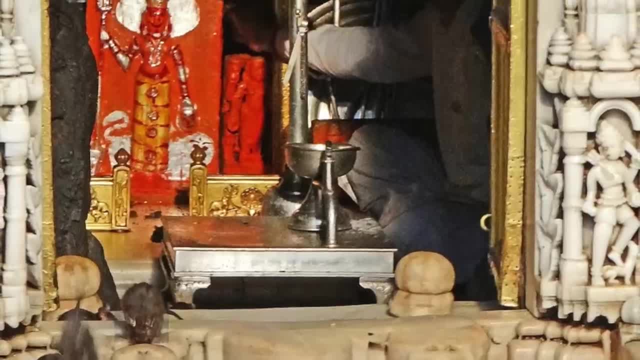 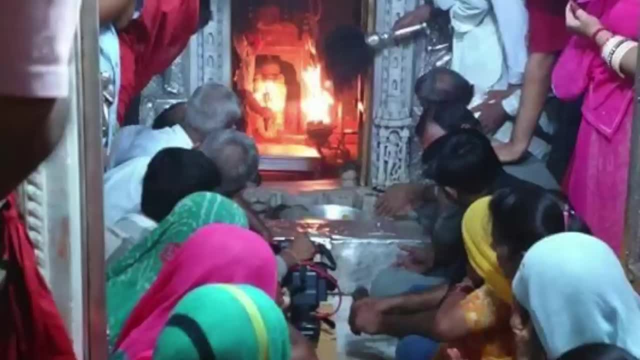 Yama first refused but eventually relented, permitting Karni Mata's son and all of her male children to be reincarnated as rats. Eating food that has been nibbled on by one of these rats is considered a high honor, The Taj Mahal. Less than 200 kilometers away is the Taj Mahal. It was called the Taj Mahal because it was the place where the people of India lived and lived. The Taj Mahal was built in the 18th century. It was built in the 18th century. The Taj Mahal was built in the 18th century. 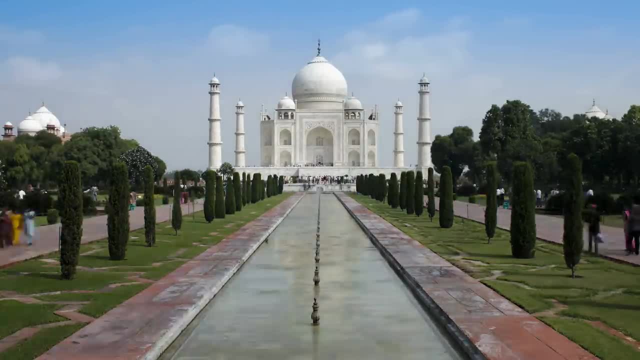 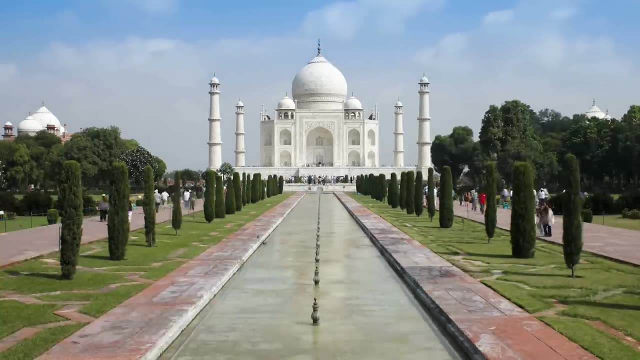 Hall. It was commissioned in 1632 and completed in its entirety in 1653.. It is estimated that at the time to have cost around 32 million rupees, which in 2021 would be around 70 million rupees, or just over 900 million US dollars. 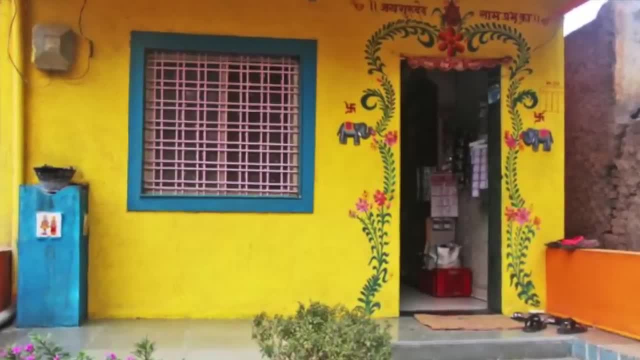 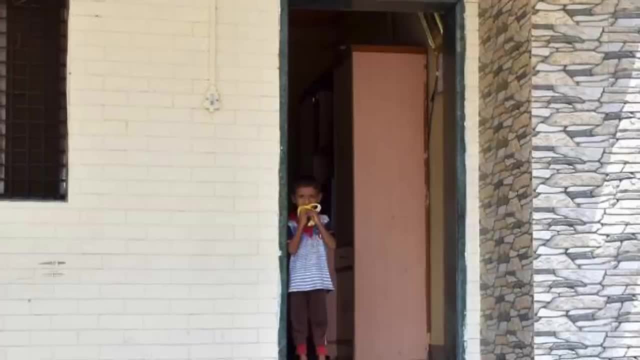 A village in India named Shani Shingnapur has no doors on any of their homes, only door frames. Despite this, there have been next to no reports of theft. There has not been an official recording of a criminal act for almost 400 years. 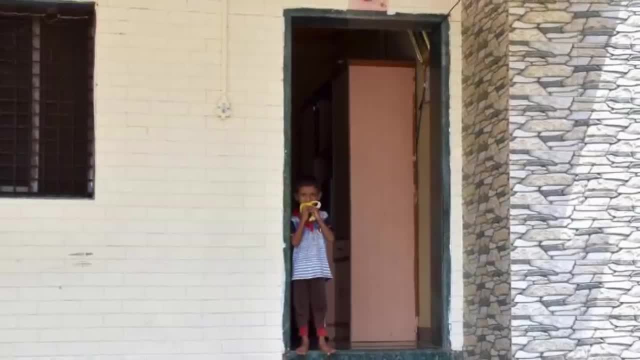 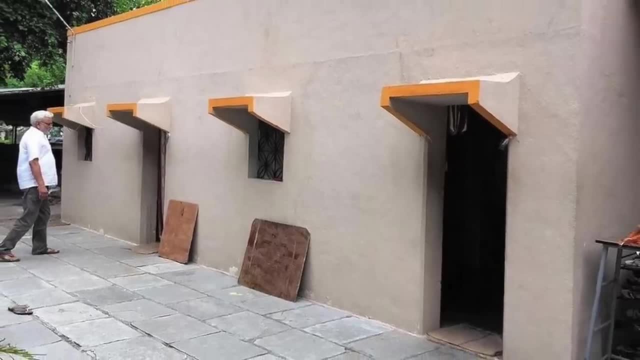 although there has been two thefts reported, once in 2010 by a tourist that claimed items were stolen from his car, and a second incident in 2011 involving gold ornaments. However, the local villagers claim that both incidents took place outside of the village. 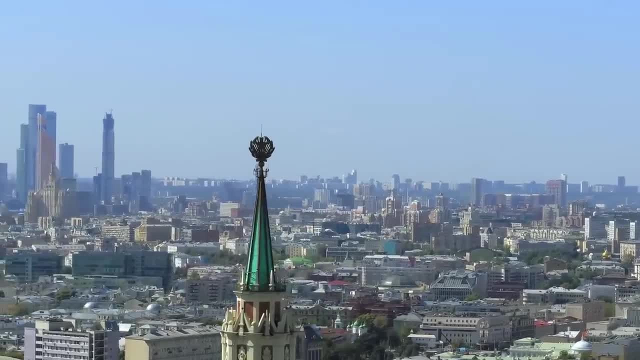 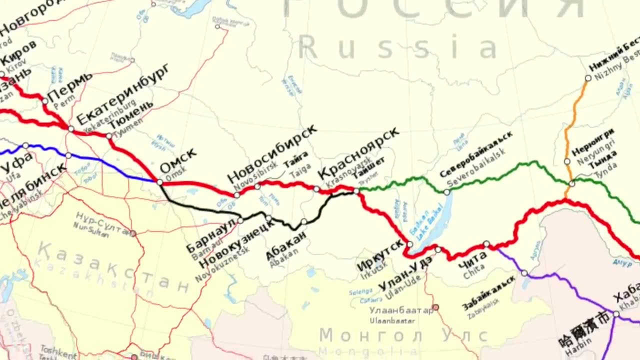 Moscow, Russia, has more billionaires per capita than any other city in the world. Russia is also home to the longest railway in the world, the Trans-Siberian Railway. It stretches 9,289 kilometers or 5,772 miles. The Trans-Siberian Railway is the longest railway in the world. It stretches 9,289 kilometers or 5,772 miles. 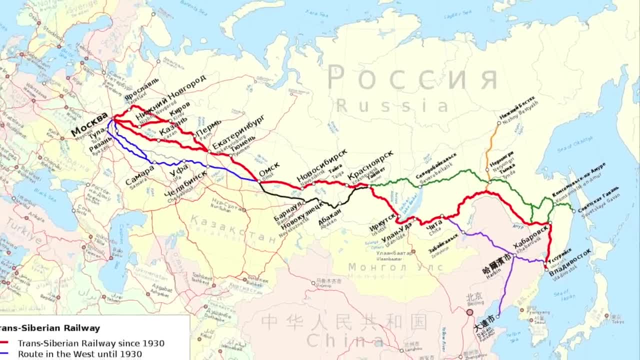 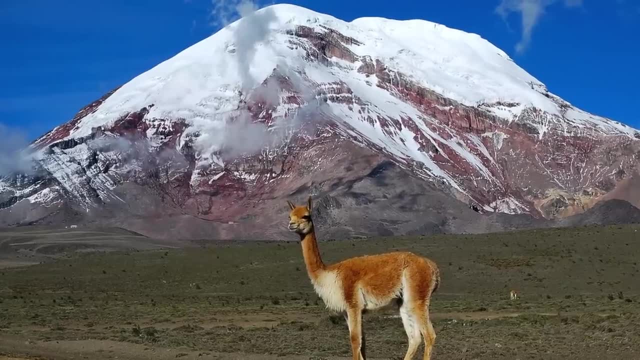 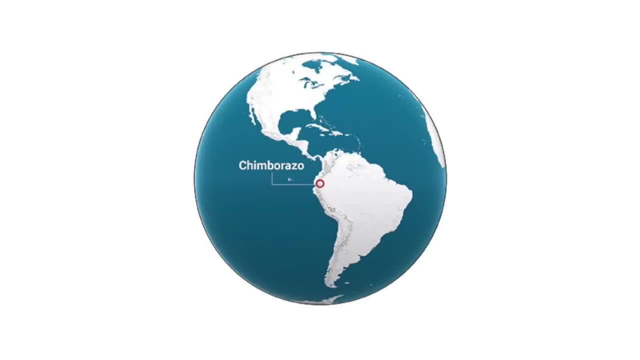 Starting with the capital of Moscow and ends at Vladivostok. Chimborazo, an inactive volcano located in Ecuador, standing at just over 20,000 feet, is the farthest point from the Earth's center, despite Mt Everest being over 29,000 feet above sea level. This is due to Chimborazo being located 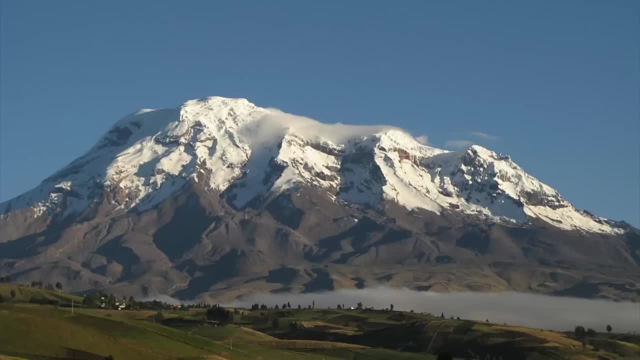 on the equatorial bulge, which occurs due to the Earth's rotation. Though Mt Everest is the tallest from sea level, Chimborazo is closer to the moon and the stars in space. Pheasant Island, a tiny island located on the Bizarroa River. 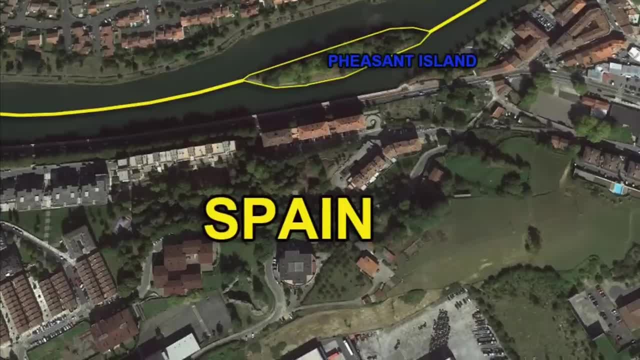 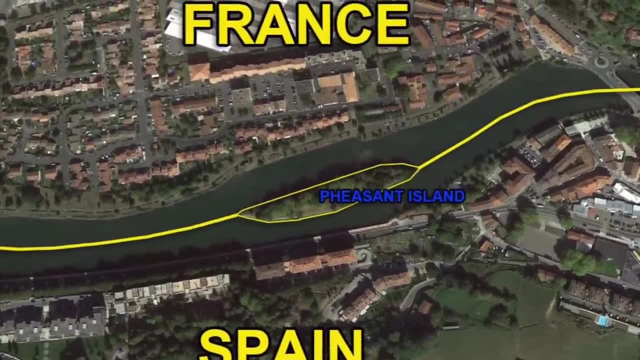 switches sovereignty every six months between France and Spain. This tradition began in 1659 as a symbol of peace between the two nations at the conclusion of the Franco-Spanish War. In 2021, for the fourth year running, Finland has come out on top as the happiest country on Earth. 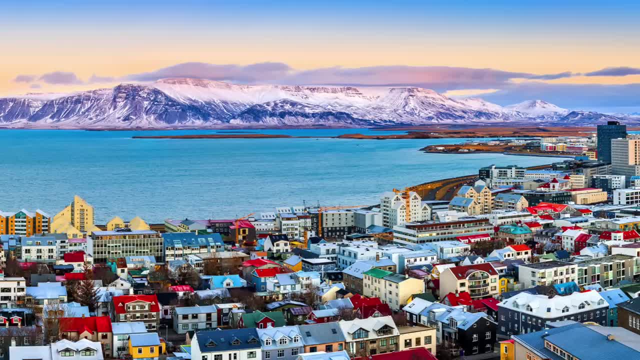 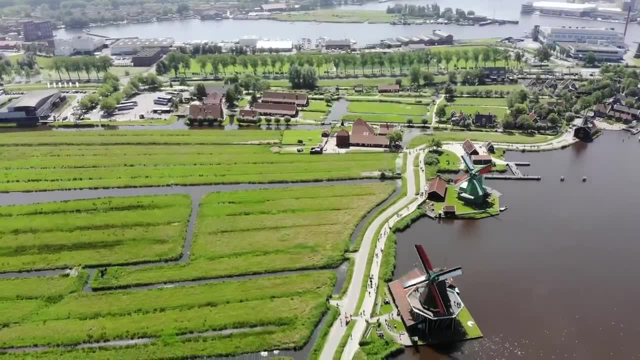 in the annual list powered by data from the Gallup World Poll, with Iceland, Denmark, Switzerland and the Netherlands following in second, third, fourth and fifth places. The entire country of Liechtenstein could be rented for $70,000 a night in the 2010s. 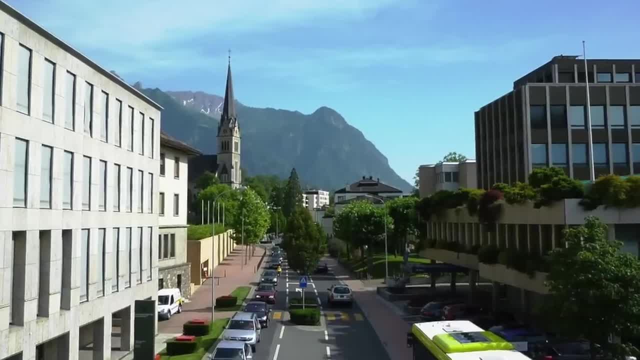 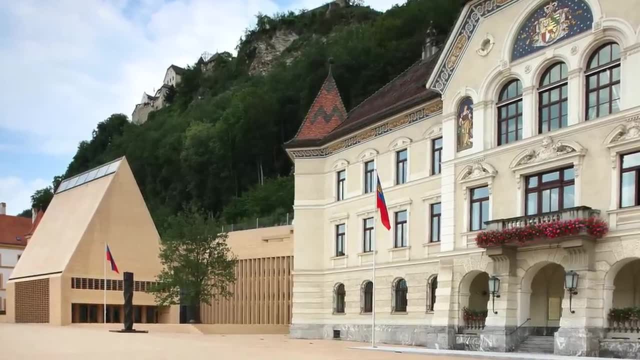 This included customized street signs, temporary currency and hanging out with the monarchy. Snoop Dogg before had asked to rent the country for a music video, but the government was unprepared. Sri Lanka was not an island until 1480, when a cyclone broke. 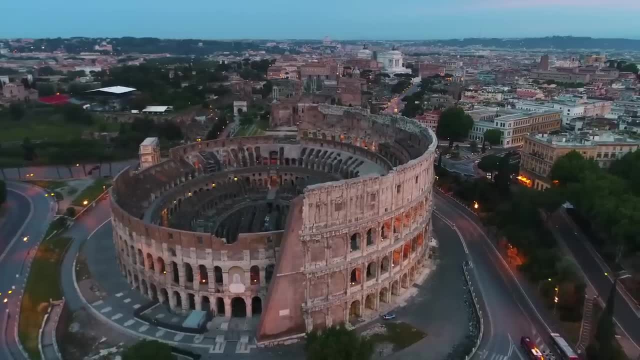 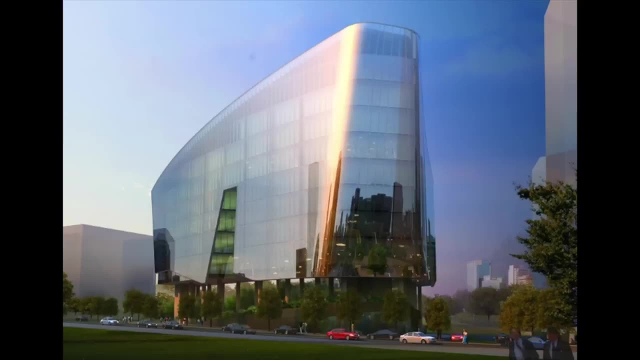 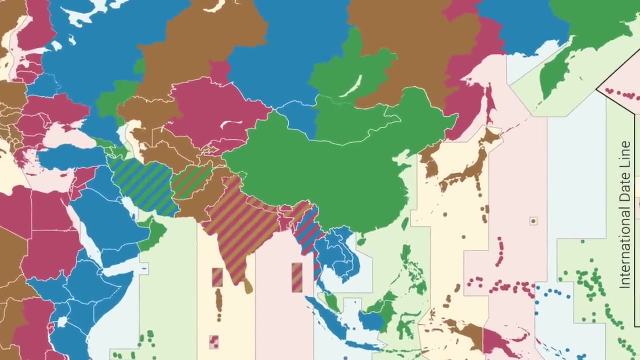 the land bridge connecting it to modern-day India. Italy has 55 UNESCO World Heritage Sites, the most of any country. Singapore is home to a Lucasfilm facility that was inspired by the Star Wars sand crawler. Though China is about the same size as the continental USA, it only has one official. 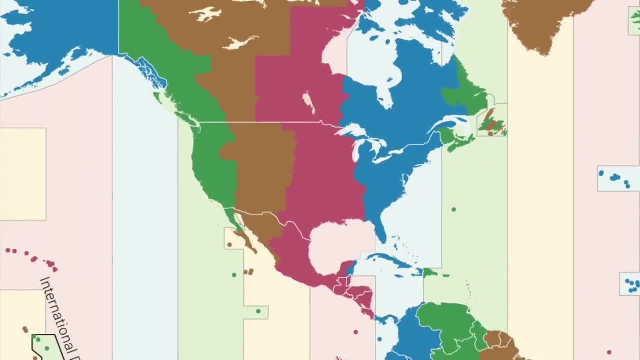 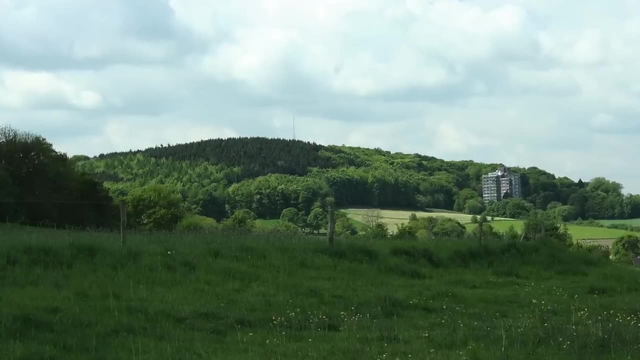 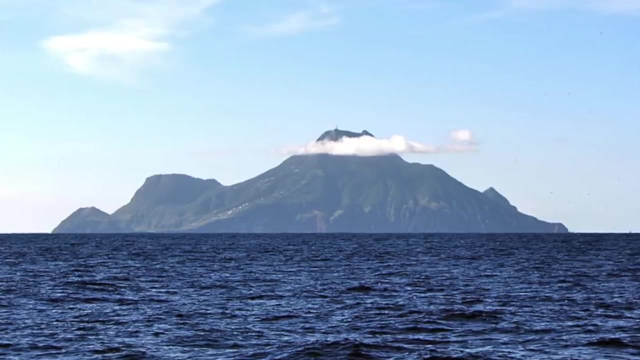 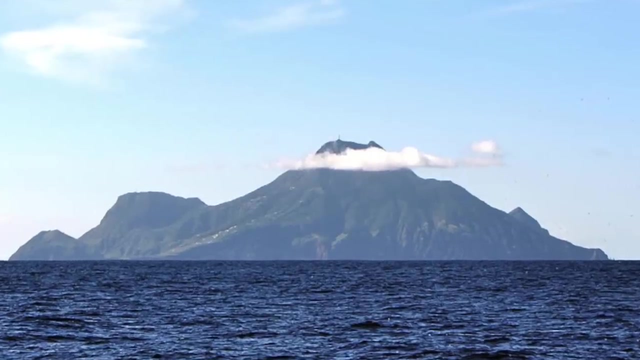 time zone, Continental United States has four. China also produces at least 45 billion chopsticks each year. The tallest point within the Netherlands proper is only 322 meters or 1,058 feet. However, the kingdom of the Netherlands is 887 meters or 2,910 feet, and is located in the Caribbean. 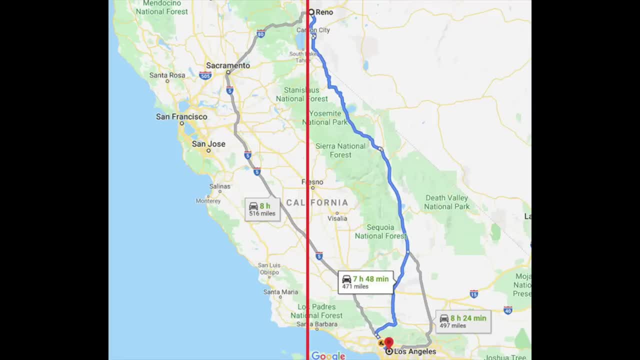 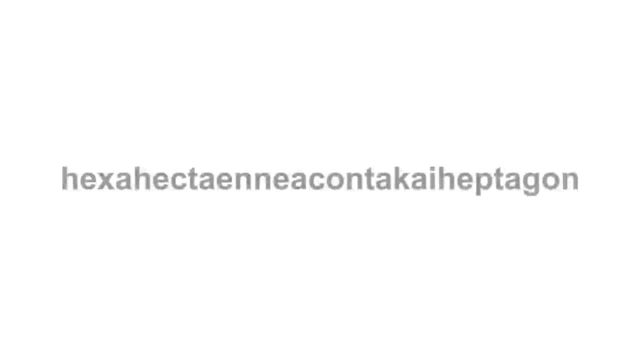 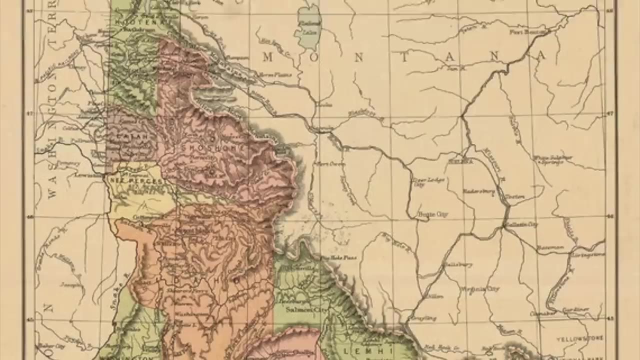 Reno. Nevada is farther west than Los Angeles, California. Colorado doesn't have four sides, but 697, meaning it's not a rectangle but a. I'm not even going to try to pronounce this. The name Idaho is a made-up word. It was first suggested to Congress by a man named George. 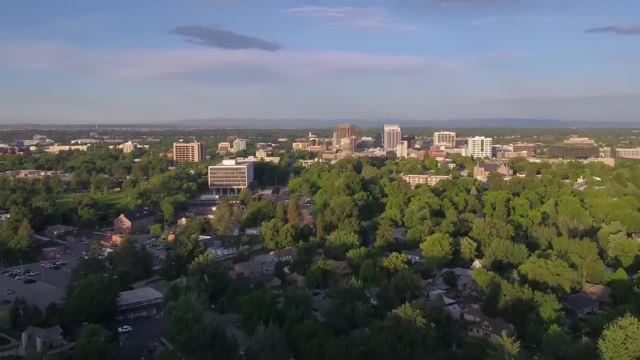 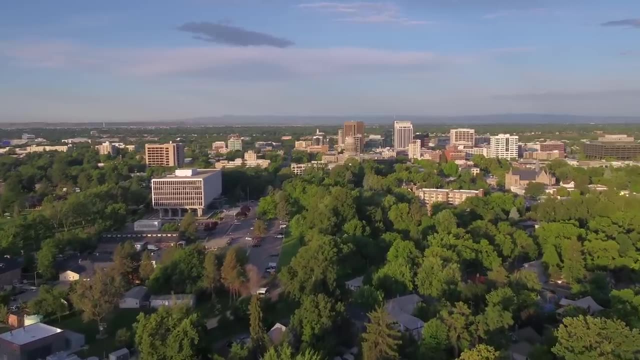 Willing. Willing claimed that the name was derived from a Shoshone term, meaning the sun comes from the mountains or gem of the mountains, But it was revealed later that there was no such term and Willing claimed that he had been inspired to coin the name when 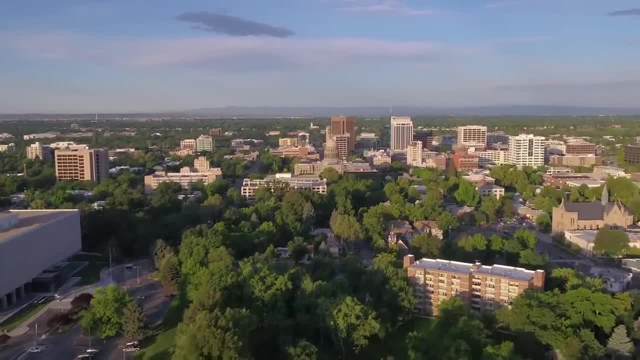 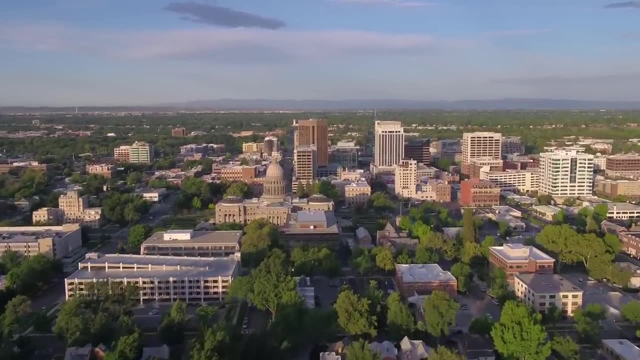 he met a little girl named Ida. Since the name appeared to be fabricated, the US Congress ultimately decided to name the area Colorado Territory, But it was too late. By the time this decision was made, the name was being used throughout the region. 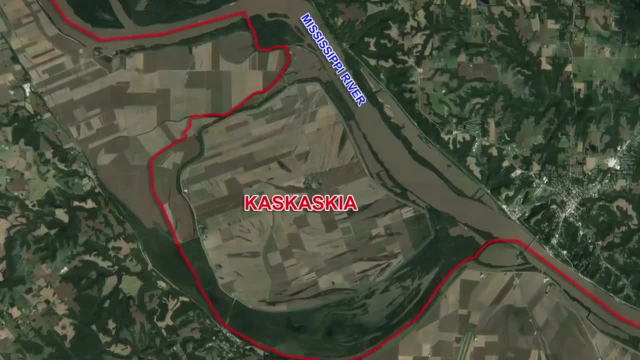 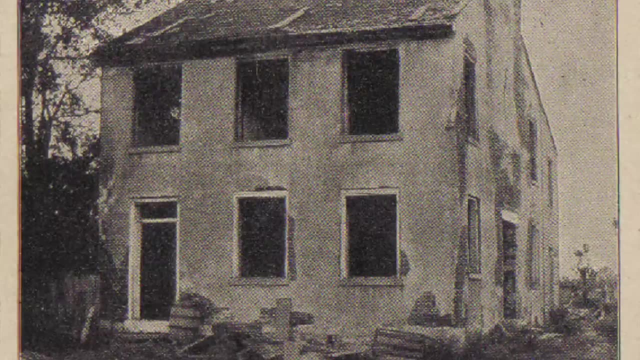 Kaskaskia, Illinois, the state's first capital, is the only known town in Illinois west of the Mississippi River. Kaskaskia, Illinois is the only known town in Illinois west of the Mississippi River, but it didn't used to be. Changes in the river's direction and depth destroyed the town with. 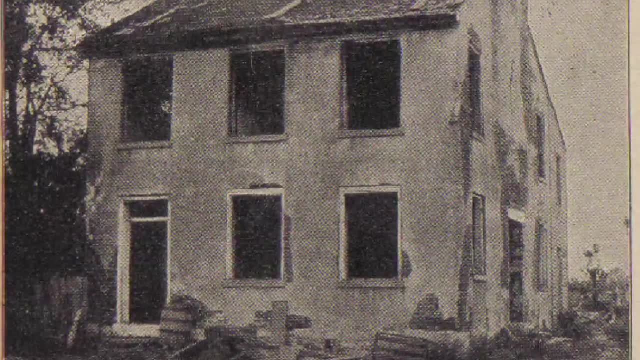 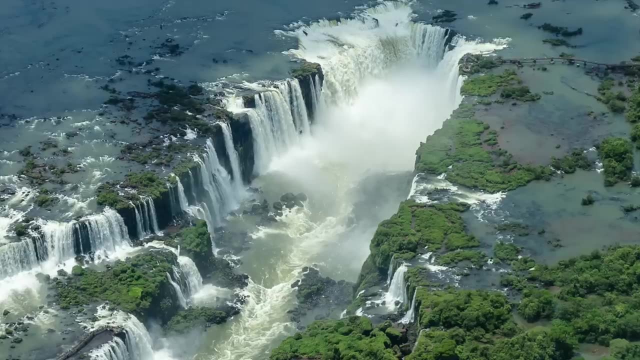 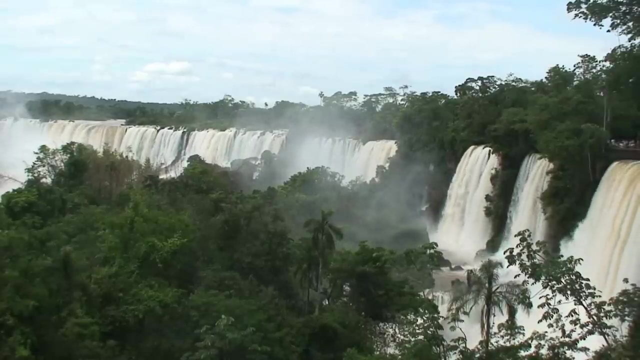 floods. What was left was cut off from the mainland Illinois. In 1818, over 7,000 people lived in Kaskaskia. By 2000, it was nine. Brazil shares the Iguazu Falls, the largest waterfall system in the world, with Argentina. There are 275 waterfalls in this waterfall system. 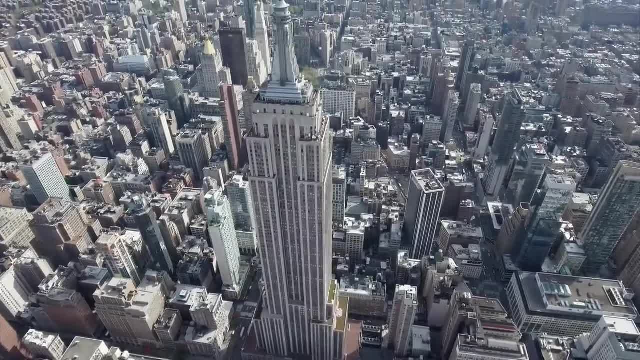 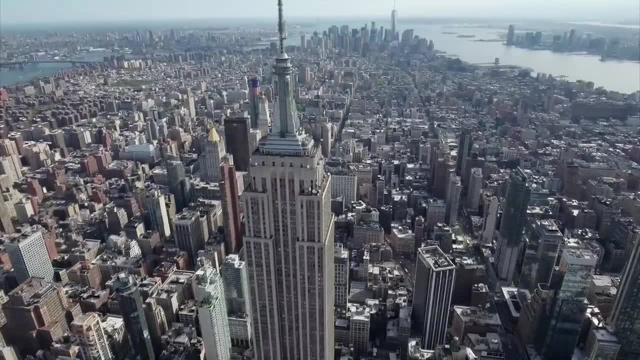 New York City is home to multiple former tallest buildings in the world, The Empire State Building being one of them. It stands at 443 meters tall, It includes 102 floors and 73 elevators, And it was constructed in 1930.. It lost its status as the tallest. 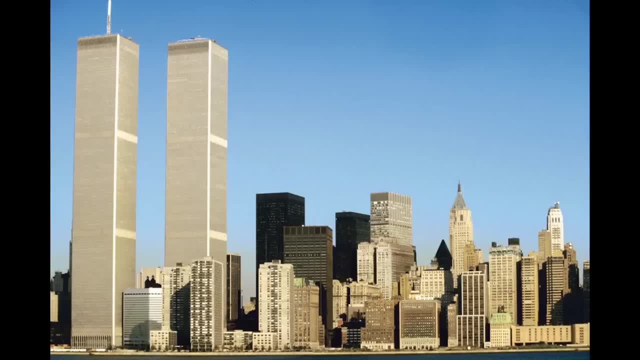 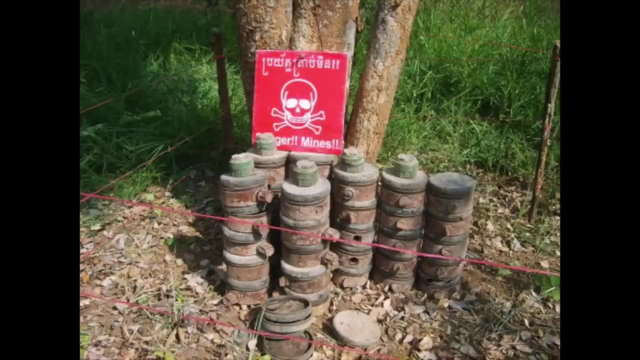 building in the world in 1971, when the World Trade Center was built. Landmines pose a major threat in Cambodia, especially in rural areas. The nearly three decades of war that raged in the country in the 60s through the 80s left vast parts of the nation. 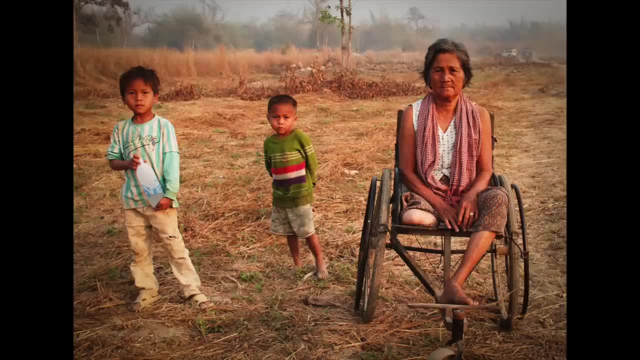 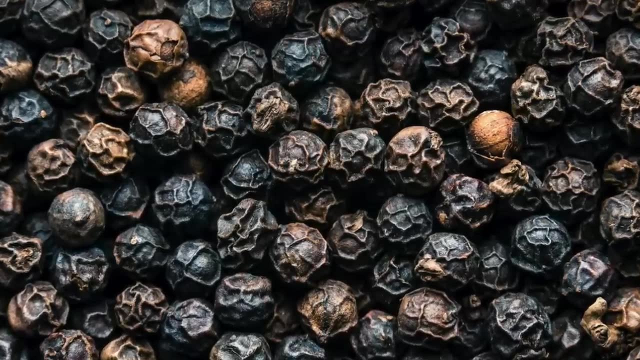 riddled with millions of these landmines and other explosives yet to be removed, Producing 24% of the world's total in 2019,. Vietnam is the world's largest exporter of pepper. Thailand is home to the largest gold Buddha statue in the world. 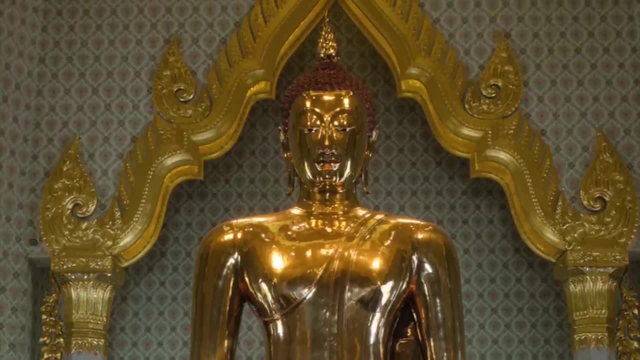 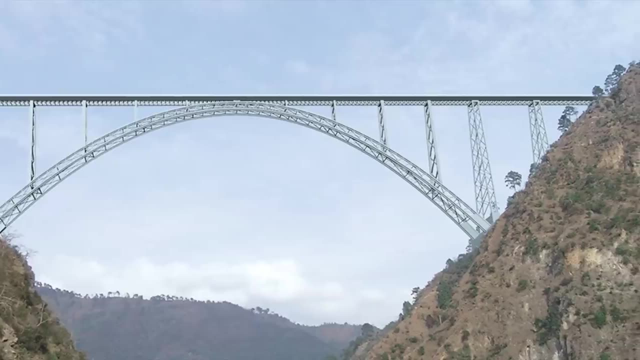 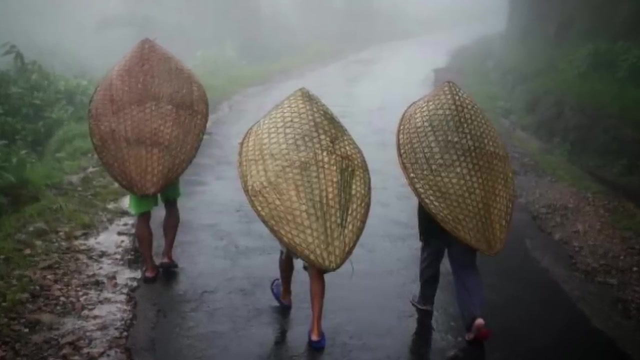 The statue is three meters tall and weighs five and a half thousand kilograms. The Chenab Bridge, located in India, is the highest rail bridge in the world, expanding 1,178 feet above the water. It is also home to one of the world's tallest buildings in the world, which is located in 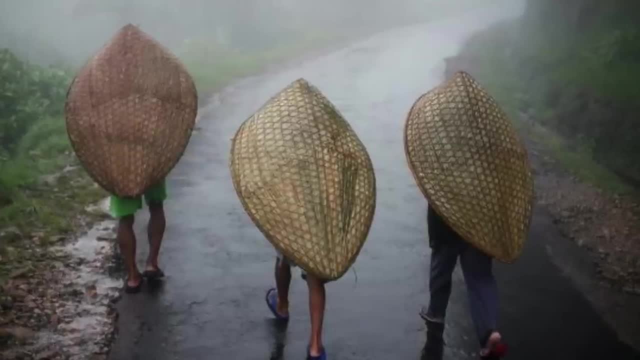 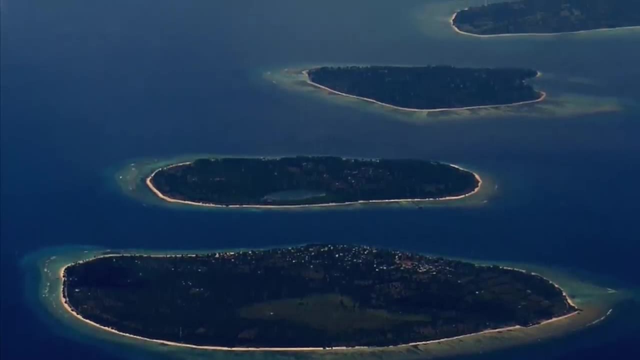 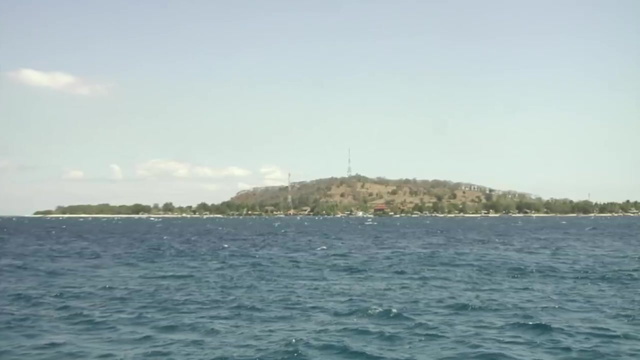 India is the world's wettest place on earth- Meghalaya, with about 11,873 milliliters of rain annually. There are over 20,000 islands in Southeast Asia, which includes an archipelago of three small islands in Indonesia called the Gili Islands, which is a misnomer, because Gili 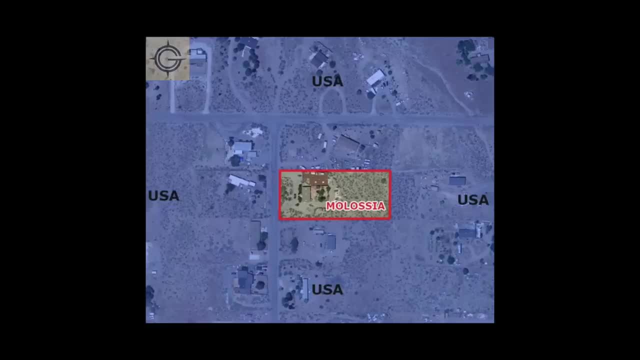 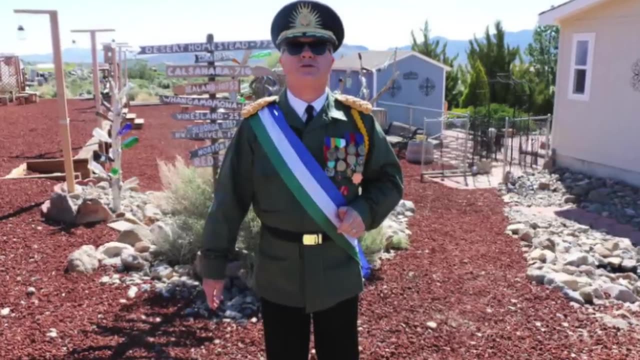 by itself simply means small island in the local language, Sasak, The micro-nation. the Republic of Malasia is a major part of the world's most popular country. The country was founded in 1999.. Its currency is tied to the value of Pillsbury Cookie Dough and it is currently at war with. 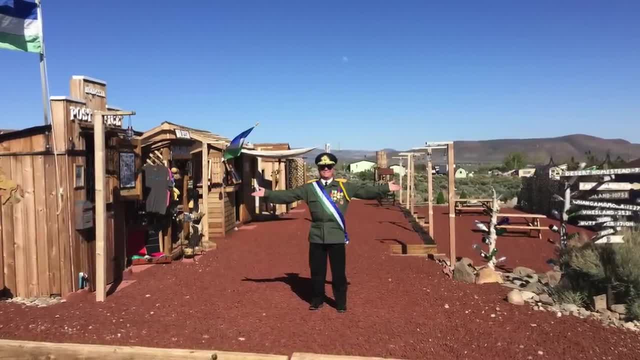 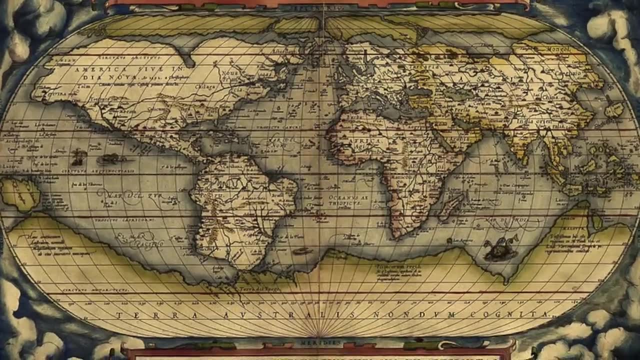 East Germany. It is also generous enough to provide foreign aid to the United States, though the United States claims this aid is actually just taxes and they refuse to recognize the Republic of Malasia as sovereign. Maps between the 15th and 18th century would often